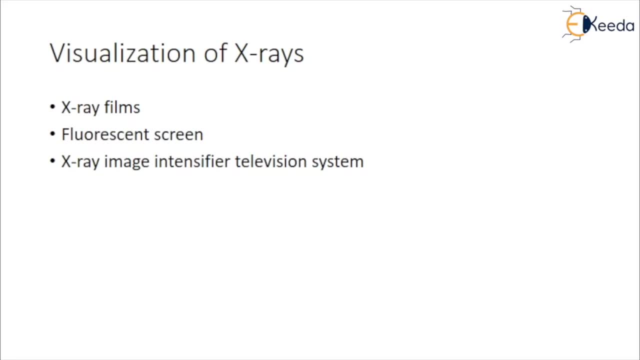 television system consists of a large evacuated glass tube with an input screen diameter ranging from 15 to 32 cm. The input screen converts the X-ray image into a light image. The light image thus produced is transmitted through the glass of the tube to a photocathode, which 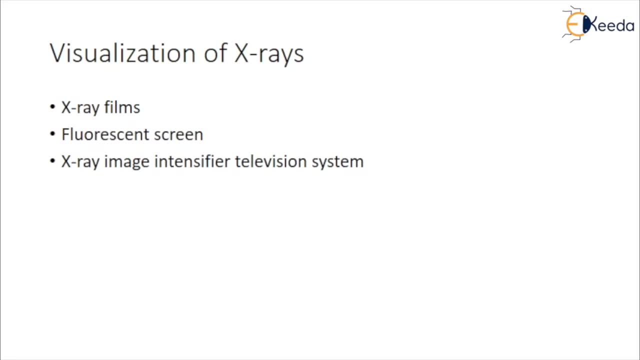 converts the light image to an equivalent electron image. The image intensification takes place because of the very small output screen size and the electron magnification in the tube. The X-ray quanta, after getting converted to a light quanta, falls on the photocathode, in which the light quanta produce electrons under the influence. 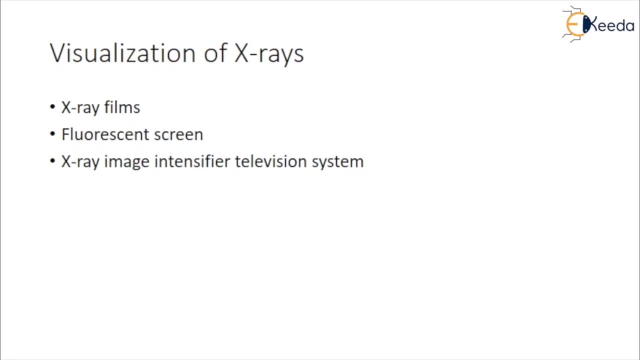 of an electric wave. The electrons are emitted from the photocathode and accelerated towards the output of phosphor while being focused by the electrostatic lane system. The electrons impeaching with the high kinetic energy on this screen produce light quanta, resulting in a much brighter and minified output image. 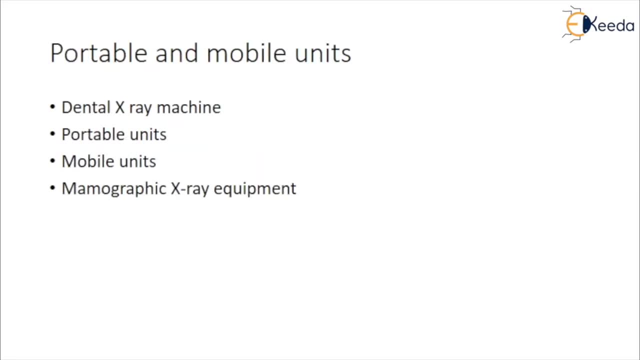 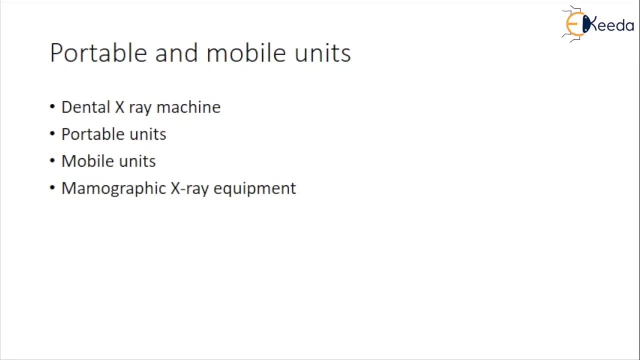 location of the teeth. The X-ray machine uses only the value. the scoop pipes are placed from the tube of theesser being to detect the location of the teeth. The device is designed for X-ray machines to detect the highly Auchan treatments ف, Uncle III. 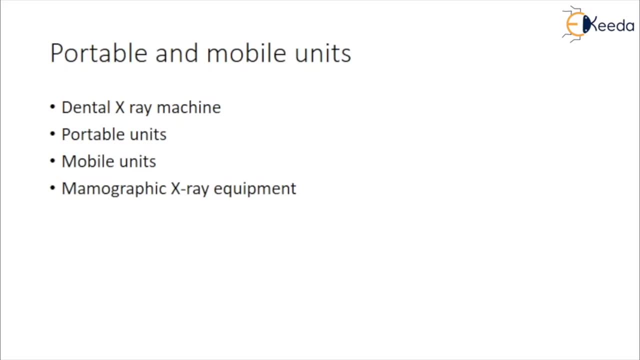 There is no need to go to the X-ray department duringragtions. The X-ray ultrasound machine works. MEMBER INDI Doesn't have to be replaced while using it. The camera Mir竿 is very easy to detect fatrichious lesions from the tooth. 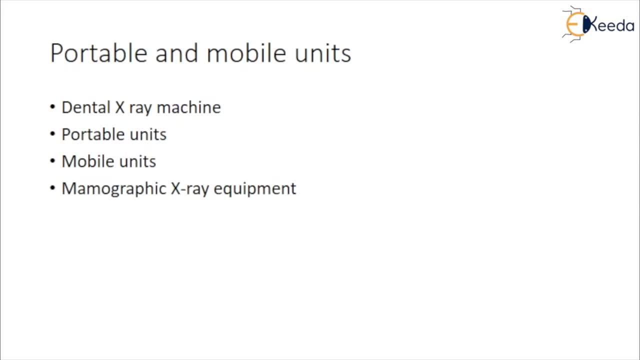 noticed有一. When the patient is too ill to the hospital, seriously ill at home, undergoing surgery in the theatre, need arises to wear X-ray equipment which can be moved to the patient, rather than patient moving to the X-ray machine. A portable unit is so designed that it can be dismantled, packed into a small case and conveniently carried to the site. 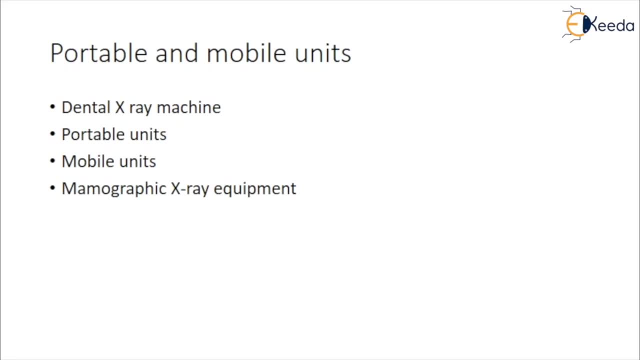 The tube head is so constructed that the X-ray tube and a high-voltage generator are exposed in one earth metal tank filled with the oil. The X-ray is usually a small stationary anode type, operating in a self-rectifying mode, connected directly across the secondary winding of the transformer. 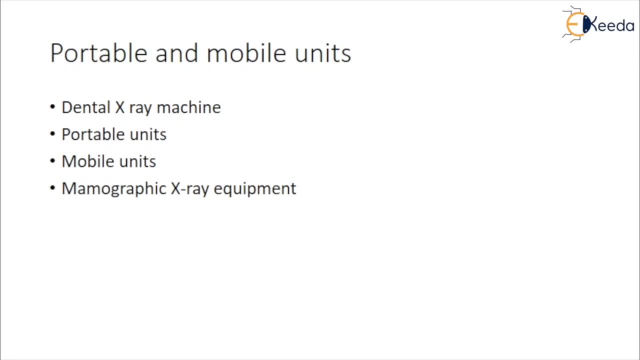 The only connection required from the control desk is for the low-voltage supply. The controls provided are fairly limited and include a main voltage compensator. Comparatively, the X-ray tube and the high-voltage generator are used for the low-voltage supply. 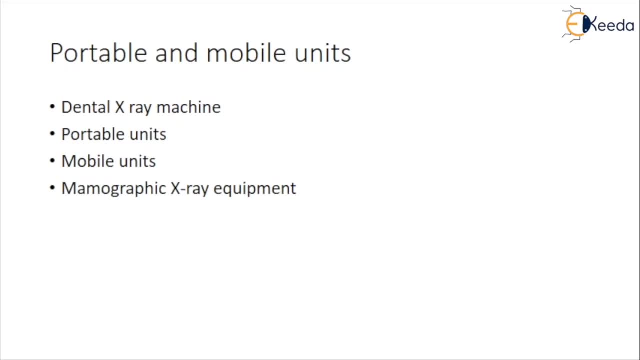 The X-ray tube and the high-voltage generator are used for the low-voltage supply. A portable unit has a combined 1 kV current switch and a time selector Unit is designed to be used on the domestic supply. The current must be limited to 15A. 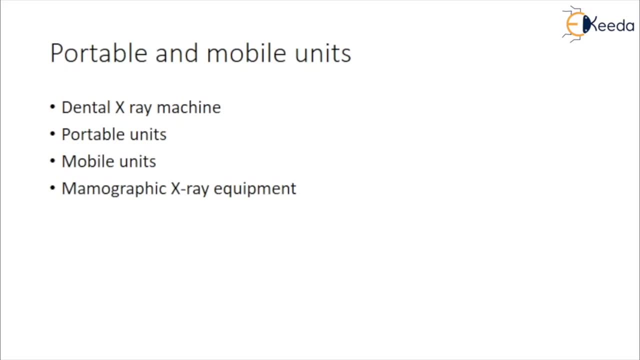 Maximum radiographic output for portable units is in the range of 15-20 mA at 90-95 kV. Mobile units can be much heavier than the portable units and are capable of providing higher outputs. Mobile units provide a greater selection of mA and kV values. Higher voltage generator has a full wave rectification circuit feeding. 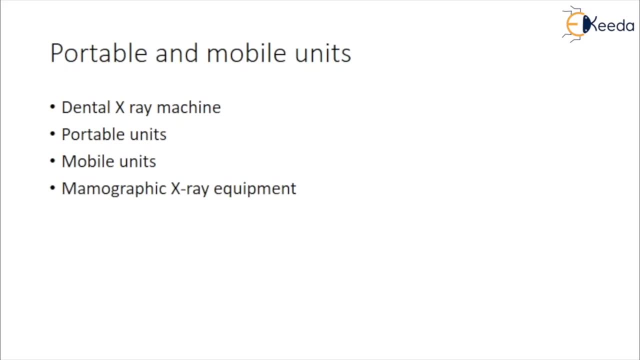 a double focus rotating anode X-ray tube. Most mobile units have a radiographic output voltage of about 300 mA and 125 kV. Mammographic S-ray equipment can either be used with special film screen or as stereo radiographic units. The units intended for a film screen use have a molybdenum. 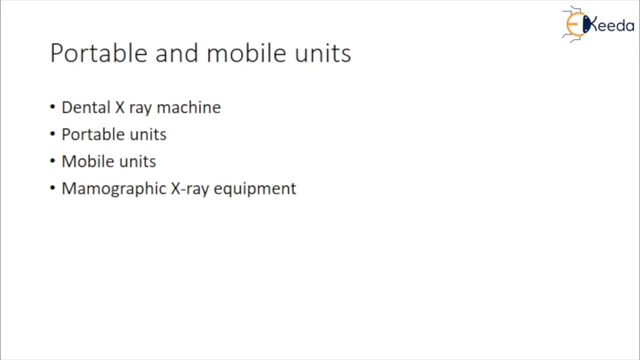 target X-ray tube with a beryllium window and 0.03 mm molybdenum filter. Radiographs are usually taken at 28 to 35 kV. Seroradiographic systems use X-ray tubes with tungsten targets about 1 mm. 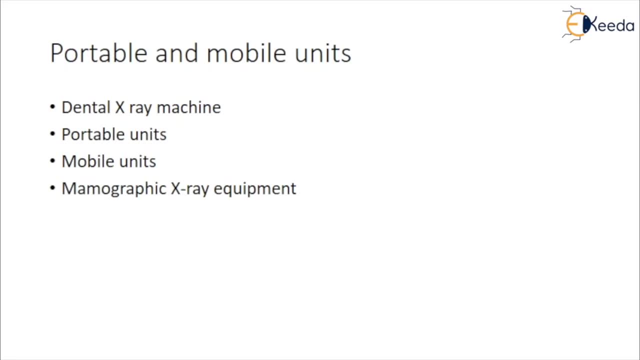 aluminum filter. Radiographs with this technique are taken at 40 to 50 kV. Both the types of mammographic units operate at low peak voltage. Physical parameters of X-ray detector: quantum efficiency. The DQE describes the efficiency of a detector: The presence of quanta for a given dose that actually contributes the 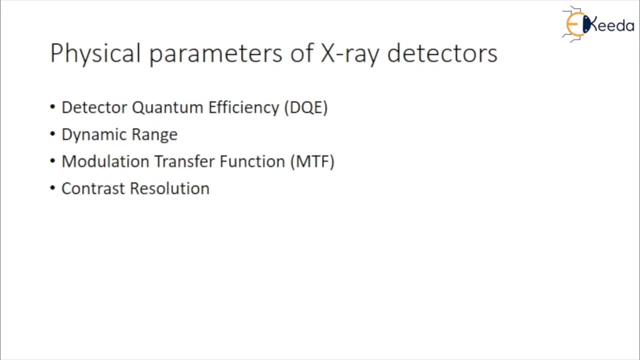 image. Its function of dose and special frequency is, by definition, effective by the various components of the system. Dynamic range: The dynamic range of the detector is the range from minimum to maximum radiation intensity that can be displayed in terms of either differences in single intensity or density differences in conventional film. 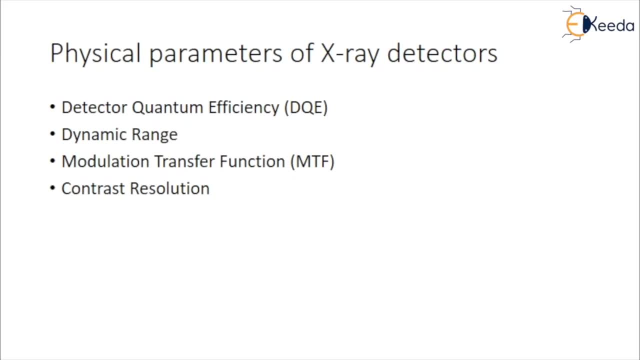 Modulation transfer function. The MTF describes the contrast of the image. component is transmitted as a function of its size or its spatial frequency. It is a function of its size or its spatial frequency. It is expressed in line pairs per millimeter Contrast resolution: It is the smallest detectable. 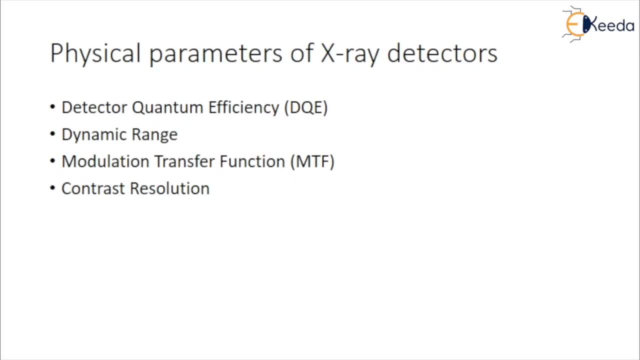 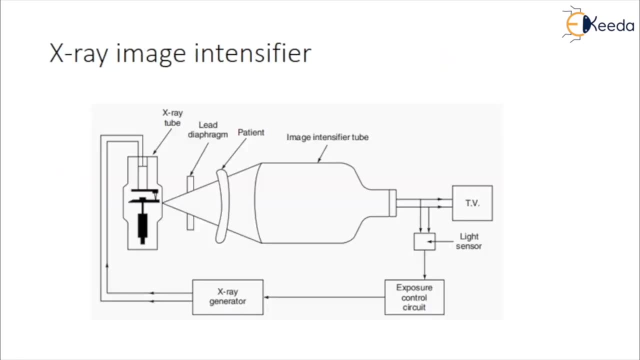 contrast for a given detail size that can be shown by imaging system with different intensity or whole dynamic range. X-ray image intensifier. The image processing for being displayed. The use of lower doses, Avoiding repeat radiography. The opening of the possibility of digital storage. 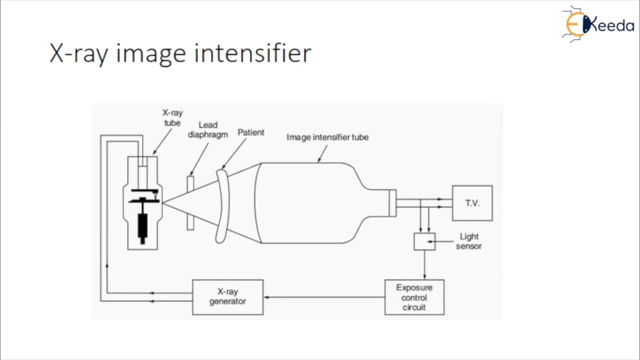 or virtual archiving and communication system or remote image viewing via tele-radiology. Digital formatted image would permit digital storage, travel, transfer and display of the X-ray images, with vast possibilities of image related processing manipulations. as much functions can be individually optimized, The application of X-ray machine intensified. 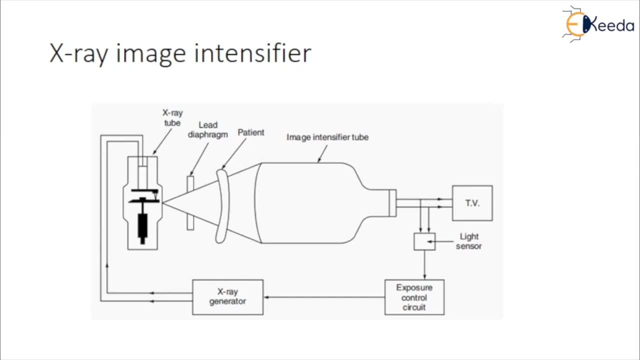 in TV systems in digital X-ray imaging evolved from their use in angiography. Angiography is a diagnostic and rapidly developing therapeutic modality concerned with the diseases of circulatory systems. Digital X-ray systems consist of the following two parts: X-ray imaging transducer or data collection, and data display, storage and processing.